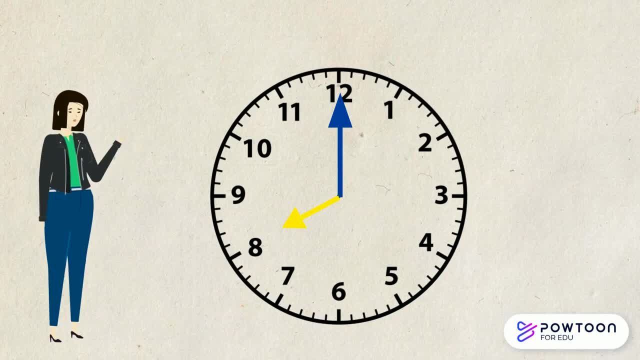 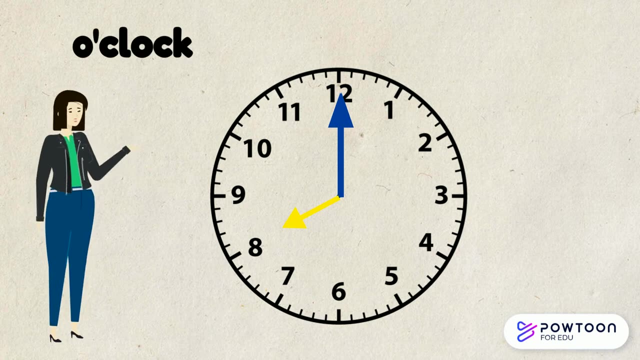 let's try one more. have a look at these hands carefully. what time does this clock show? let's see how you did. the long hand is pointing to the 12, so we know that it is o'clock. the shorthand is pointing to the eight, so this means that the time reads 8: 0 o'clock. good job. 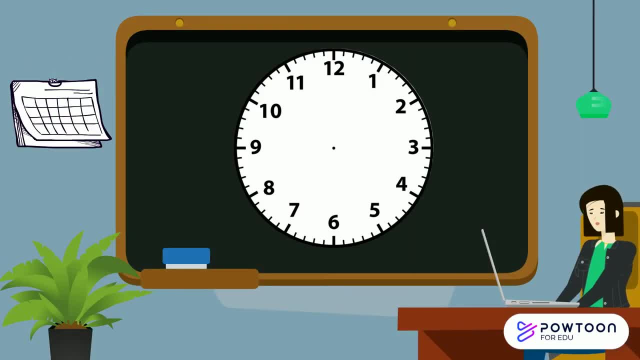 let's have a look at something new. what happens when the long hand is now pointing to the six? this means that the long hand is moved half way around the clock, so this is known as half fast. the shorthand still tells us what our hour in. You can see, this hour hand is between the 9 and the 10 because it's making its way. 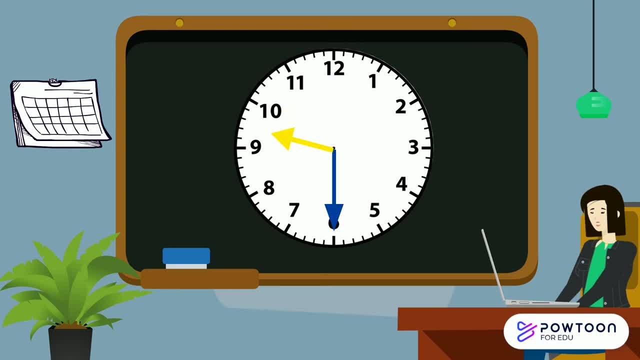 towards 10 o'clock. This time reads half past nine. Now it's your turn. What time does this clock read? Pay careful attention to where the long and the shorthand are pointing. Let's see how you did. The long hand is pointing to the 6, so we know that it is half past The. 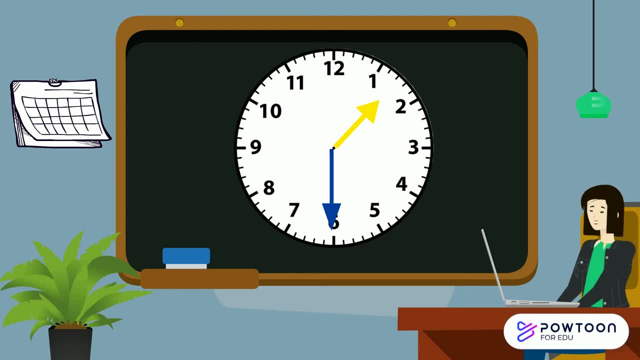 shorthand is in between the 1 and the 2.. This means it is just past one o'clock, So the time reads half past. one Good job, Let's try one more. What time does this clock read? The long hand is pointing to the 6,, so we know that it is half past. The shorthand is in between. 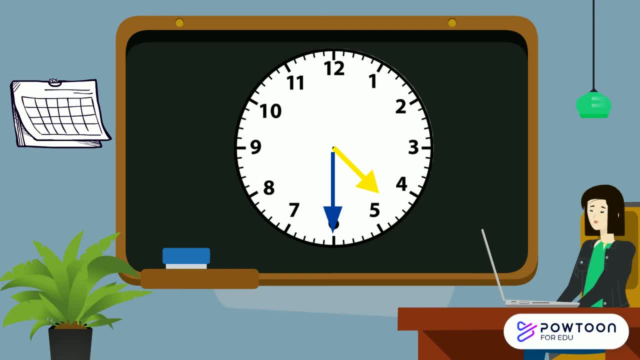 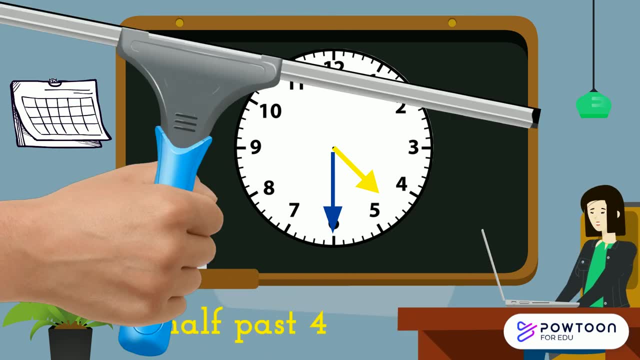 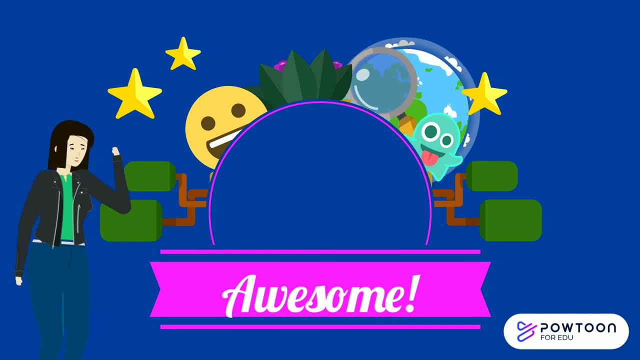 the 4 and the 5.. This means it is just past four o'clock. The time reads half past four. Good job, Awesome job. Now you know how to tell the time when it's half past and when it's o'clock. Until next time, Have fun telling the time.